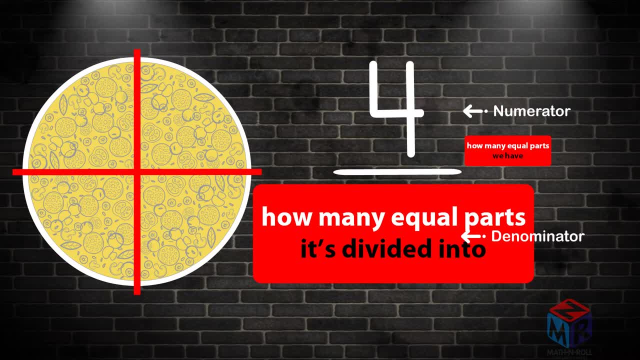 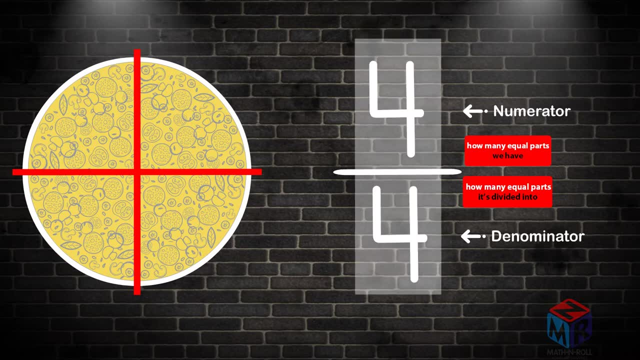 into four equal parts, so the number on the bottom will be four. We still have four of those parts, so the number on top will also be four. We have four out of four parts. The numerator is four, the denominator is also four. so 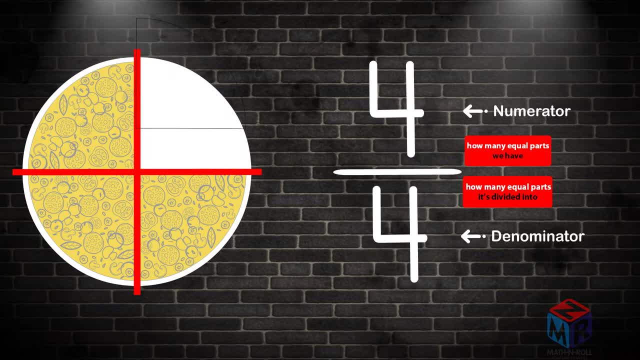 the fraction is four over four, We have the whole pizza, but what if someone came by and ate one piece? The pizza is still divided into four parts, so the bottom number, the denominator, would still be four, But we have only three of those parts left. so that means 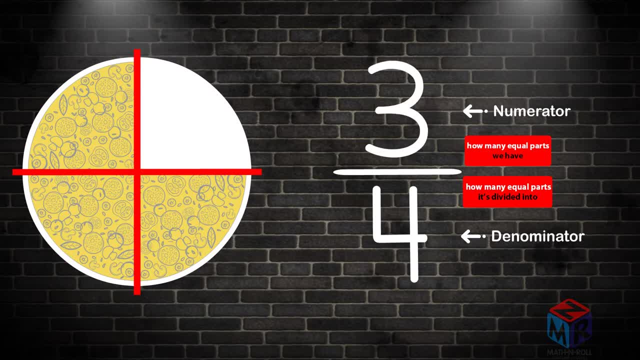 that the top number, the numerator, would change to three. So we have three over four of the pizza. The numerator is three, the denominator is four and the fraction is three over four. What if someone came by and ate one more piece? The pizza is still divided into four parts. 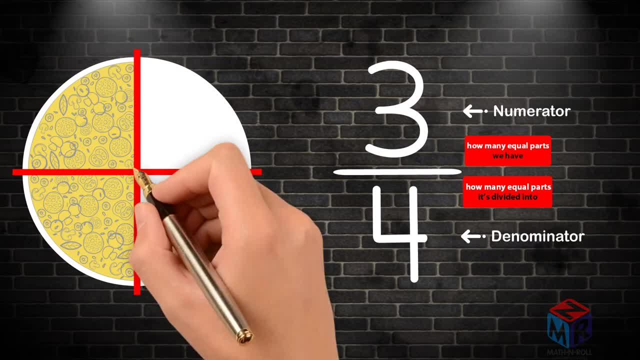 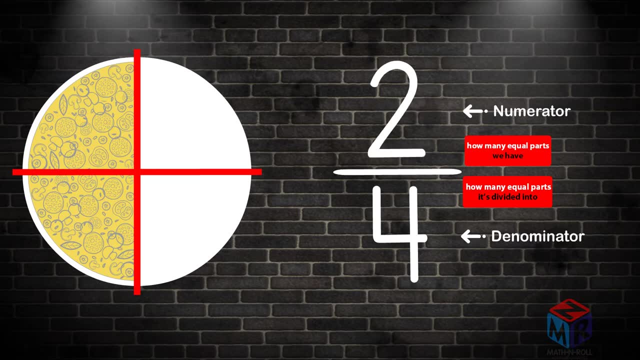 so the bottom number, the denominator, would still be four, But we only have two of those parts left. so that means that the top number, the numerator, would change to a two. So now we have two over four of the pizza. The numerator is two, the denominator is four and the fraction 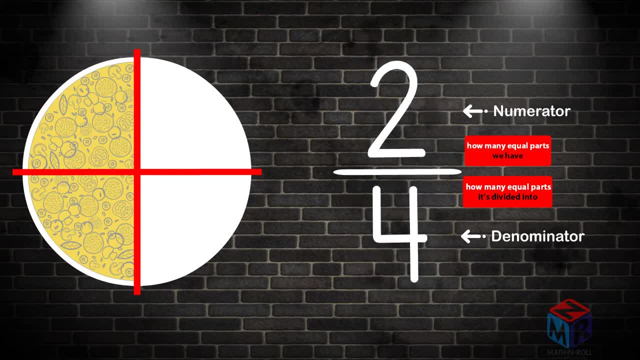 is two over four. One over four is a unit fraction. A unit fraction is a fraction whose numerator is one, So the denominator is one, the denominator is four and the fraction is two. So now we have three of those parts left. We have the whole pizza. but what if someone came by and ate one more? 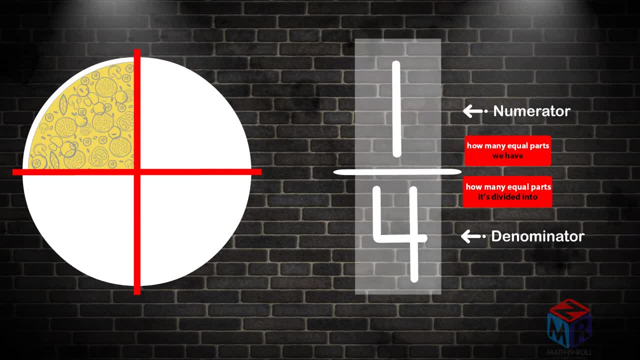 piece. The pizza is still divided into four parts, so the bottom number, the denominator, would still be four. But we only have one piece left. so that means that the top number, the numerator, would change to one. So we only have one over four of the pizza, The. 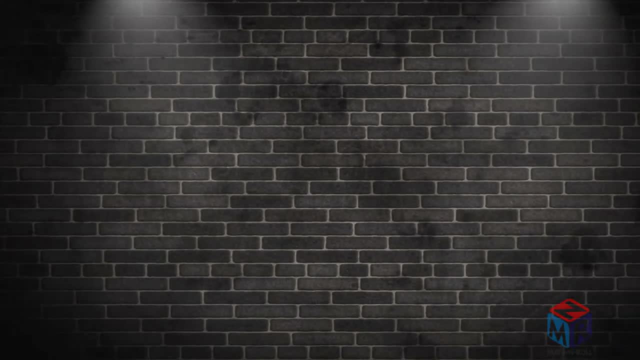 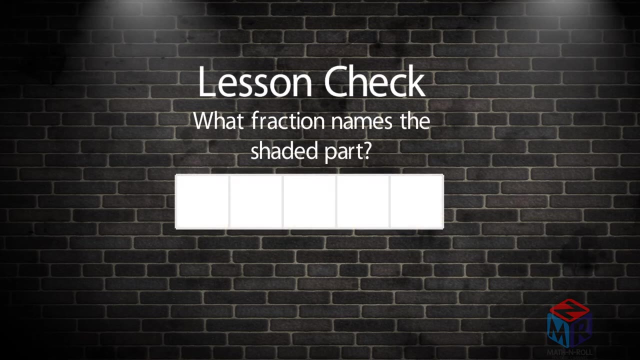 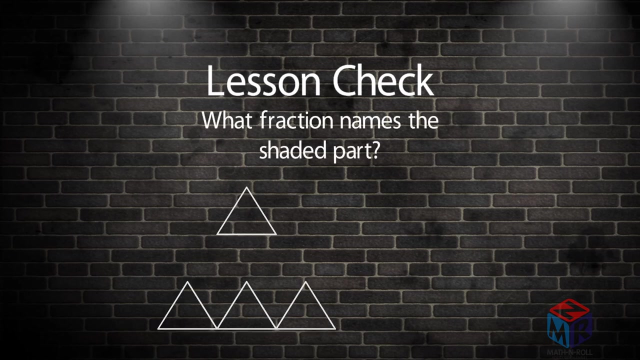 numerator is: one Lesson: check What fraction names the shaded part. Four over five: Lesson: check What fraction names the shaded part. If this video was helpful, please leave a like For more videos like this. please subscribe.